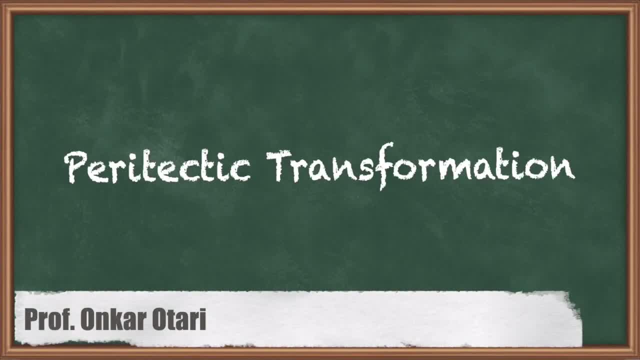 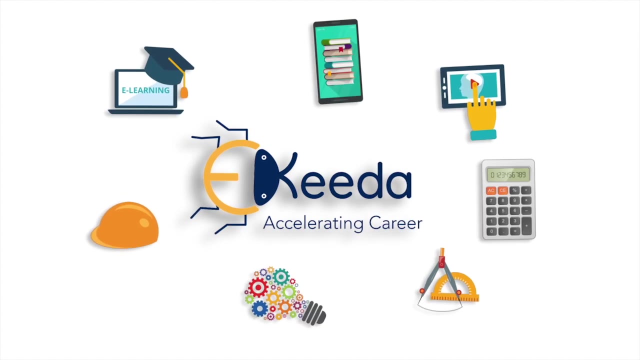 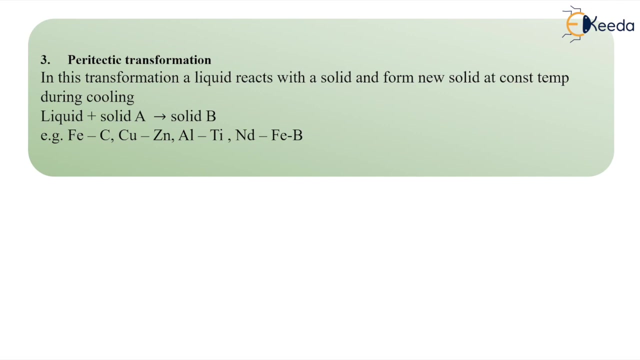 Welcome students. Now in this video we are going to talk about this peritectic transformation, or little bit in details about this peritectic reaction, dear students. So what is this peritectic reaction or this transformation? Here this liquid react with one solid. See, here liquid is going to react with the solid A and it will form the another solid, that is, the solid B. 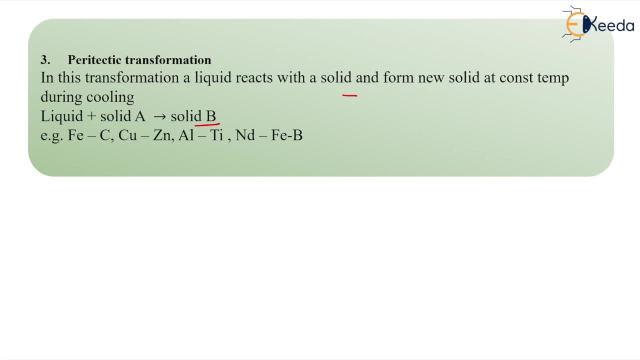 Isn't it? So what is mean by actually, peritectic reaction? So, dear students, peri is a Greek word that means around. Peri means around. That is the meaning Actually. just keep it in mind, We will come to know why it is called it as peritectic. 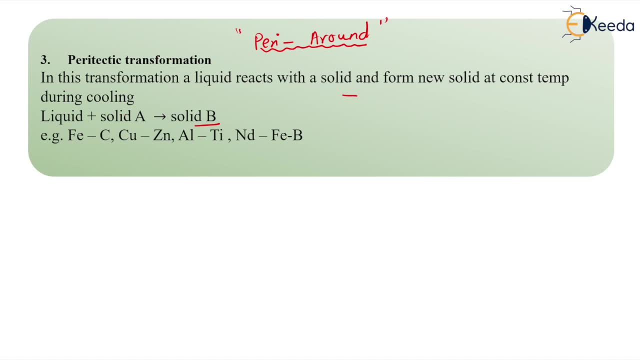 So what are the very famous examples for this reaction, dear students? We are having iron, carbon, copper, zinc, aluminum, titanium and This niadium iron and this boron. Okay, So this is the strong magnet. Actually, this is also having this peritectic transformation or peritectic reaction. 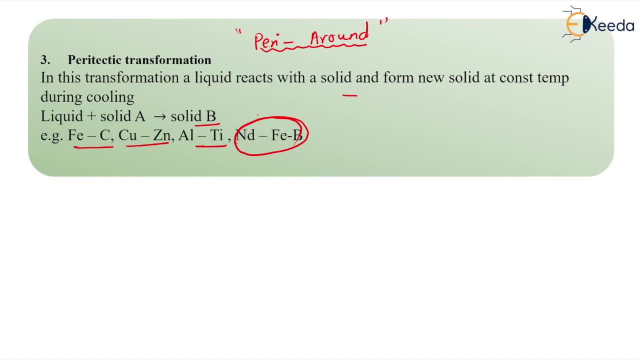 So, dear students, this copper and zinc, that is nothing but the classical brass. This is the classical brass, is the peritectic alloy, is the peritectic alloy system, That is, it is having more than five, more than five peritectic reaction. 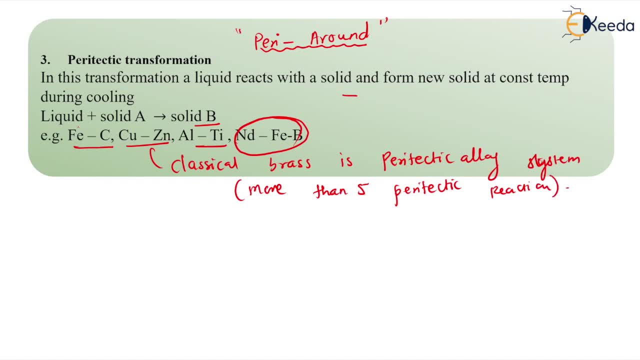 Okay And dear students, the very famous reaction in this iron carbon equilibrium diagram, that is, the reaction at the higher temperatures and the carbon percentage around 0.13%. See, at this extreme left you will be having this reaction, dear students. So this is delta, this is. 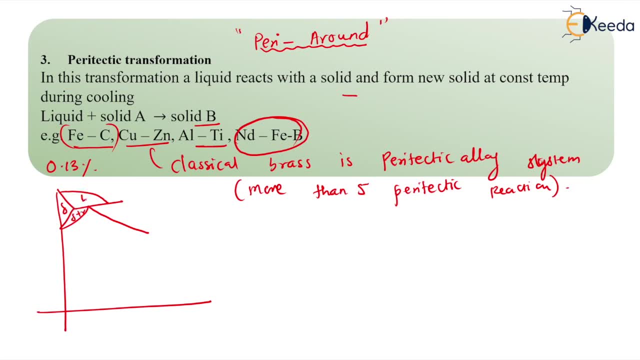 delta plus gamma. this is liquid plus delta and it will use you this gamma austenite and, of course, here is the liquid. So this is what delta plus liquid is going to for, that is delta iron plus liquid. when cooled it will go into for this gamma austenite. this 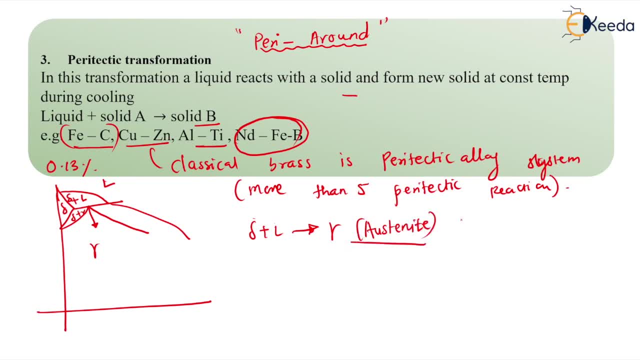 gamma austenite. So this is the peritectic reaction at dear students. 0.13 percent carbon: very, very low percentage of carbon, dear students. okay, Generally we can say that we can see these reactions in the stainless steels, okay. So, dear students, this is about. 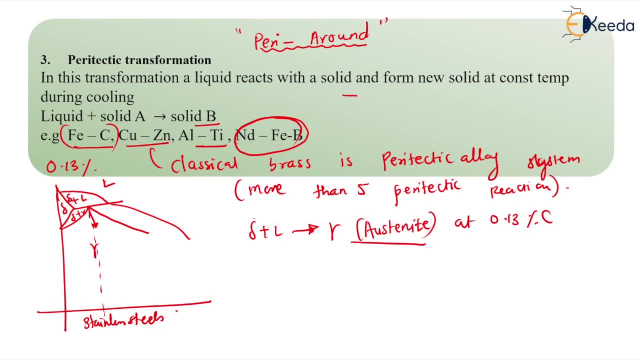 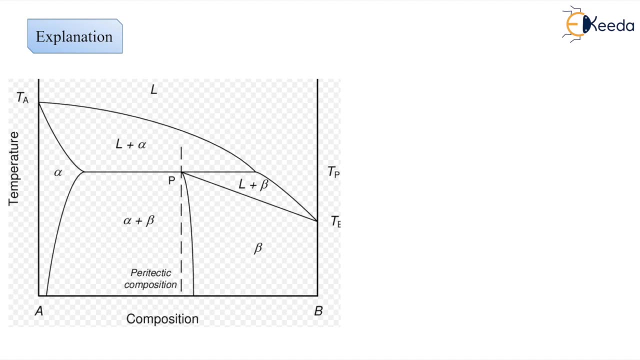 the peritectic transformation. Now, when I say the peritectic transformation, so if you look at the phase diagram, how you can able to understand whether it is a peritectic or eutectic. So definitely, dear students, when we see the diagram like this, definitely like. 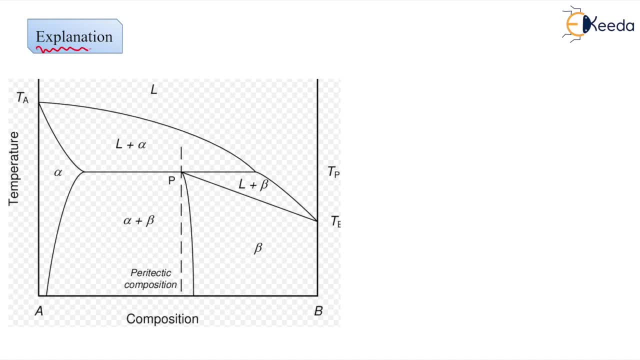 this. here we are having some detailed explanation About this peritectic transformation, dear students. So you can see here, dear students, this component A and this B. it is, of course, binary alloy system. the temperature, melting point, temperature of A, this is T A and you can see here this melting point, temperature of this. 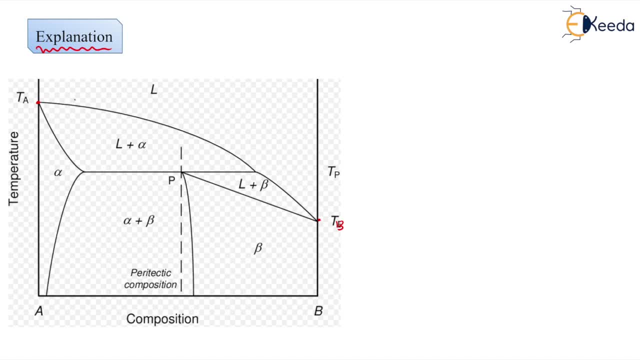 B, you can see. So whenever in the phase diagram there will be the huge difference in the temperatures of the given elements or given components, definitely you can say that there will be these peritectic reaction. So when you can say that, so when there is, when there is, 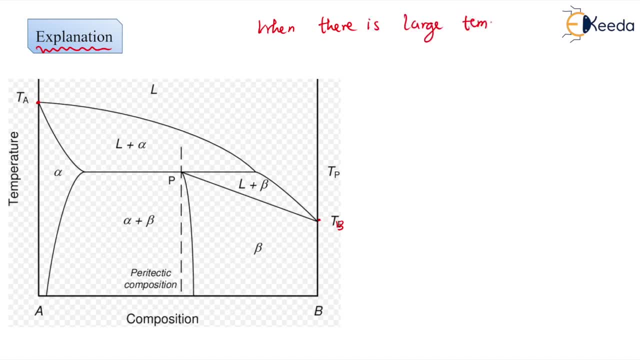 large temperature difference. large temperature difference, the temperature difference between which phase diagram? It will say peritectic phase diagram, Or you can say there will be the ~. there will be the which phase diagram? Peritectic phase diagram- Large temperature. 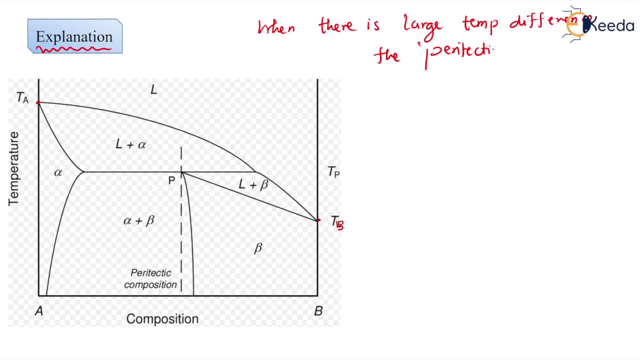 difference between this two components or elements. it will show you these peritectic phase diagram. This is, dear students. So, dear students, now, in this phase diagram, see This: of course, this liquid plus alpha, that is one liquid, seems to be onto the commission. 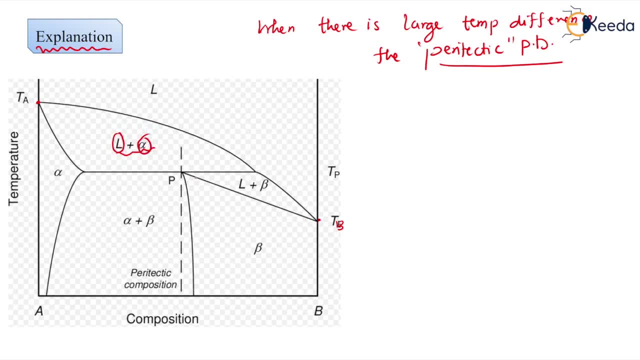 quintessential Taiwanese have shown graph. Now see a little CT. okay, So the liquid which really is react with one solid and it is going to give us what this another solid. so here, liquid react with this alpha during cooling. it will form this beta, isn't it? so this is the peritectic reaction we 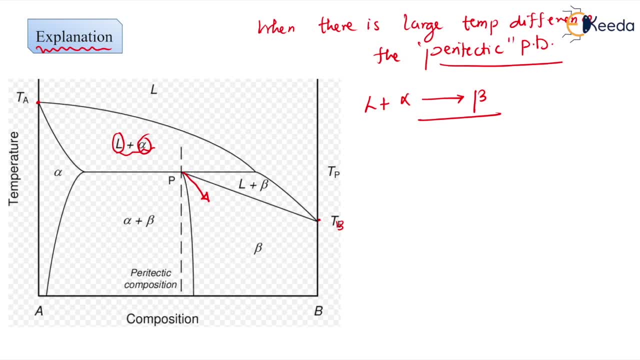 are having. so, dear student, if we see here, so how many two phase fields are here? so this is two phase field, this is two phase field and this is two phase field. so here we are having three two phase fields. how many single phase fields? how many single phase fields? one? 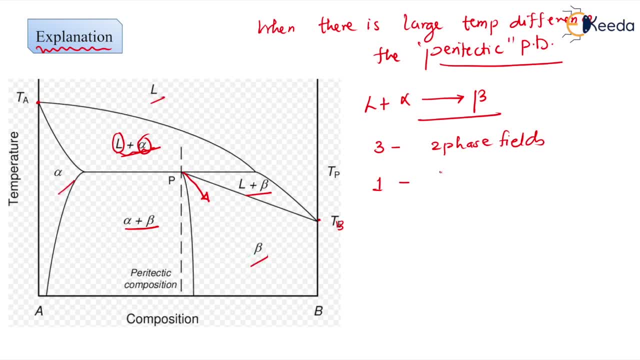 the liquid alpha and beta, that is, the three phase fields, single phase fields. okay, and when you come to this peritectic point where the peritectic reaction is going to happen, so this is the peritectic reaction is going to happen at temperature, say, i am saying that this temperature where the peritectic 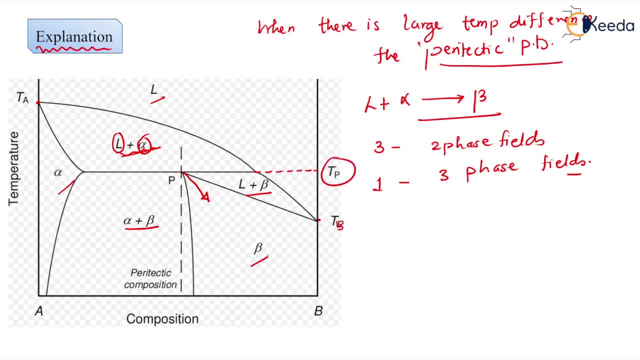 reaction is happening, that is temperature tp. okay. so, dear students, here the peritectic reaction happening, at what? this temperature tp? where this liquid plus alpha is trying to form the solid beta? at peritectic point p. this is the peritectic point p, okay, Okay. so, at the pericaptive point, dear students, if you are going to apply the phase rule or the Gibbs phase rule, so what we can write here, dear students, so how many number of phases we are going to apply the phase rule at this point? 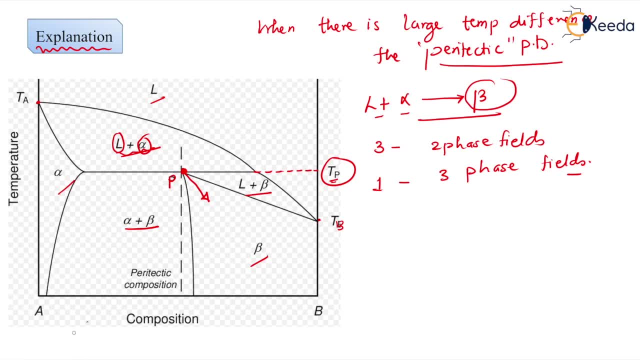 So, if I apply here. so number of phases are: how many? Number of phases, of course, 1,, 2 and 3, number of phases: 3.. How many components, dear students? Of course this is binary system, so components are 2.. 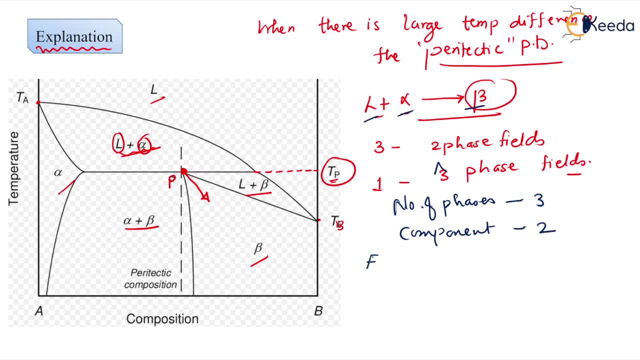 So apply these Gibbs. phase rule that is P plus F is equal to C plus 1.. We are applying the condensed phase rule. So phase rule, Phase 3 plus degree of freedom. we are going to calculate Components 2 plus So 3, 3 get cancelled, So degree of freedom will be, dear students, 0. 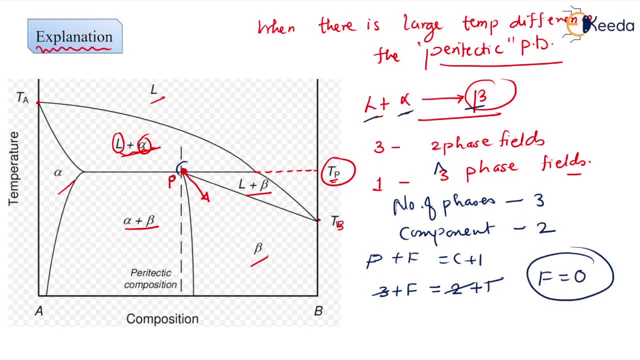 So once again you can say that, dear students, this point, the point P, is what? That is the invariant point. We cannot move from that point because as soon as we move up or down, or at the sides, definitely we will be thrown out of the 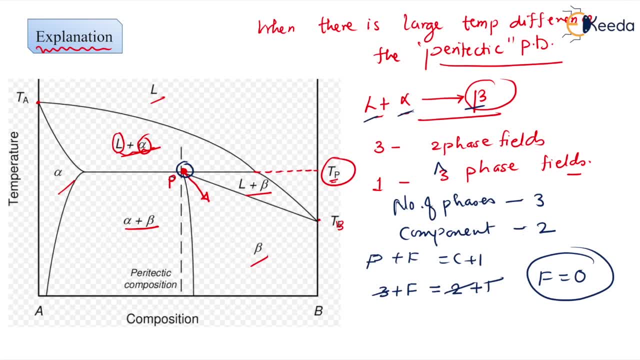 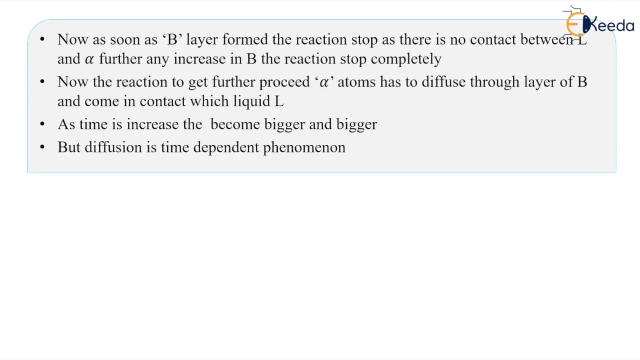 Composition, isn't it? So that is the reason why, dear students, this point P is the invariant point. So point P is invariant point where the degree of freedom is equal to 0, isn't it? Now, dear students, say, let us discuss the reaction. Let us discuss the reaction here, dear students. 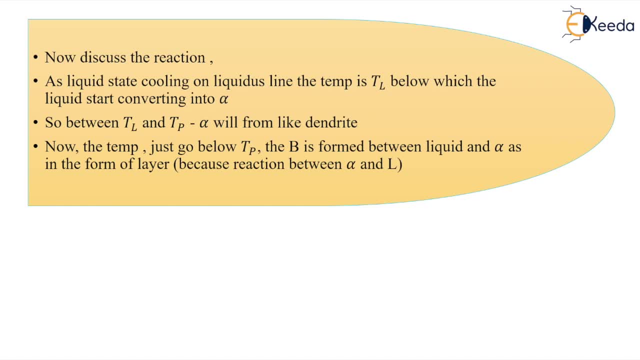 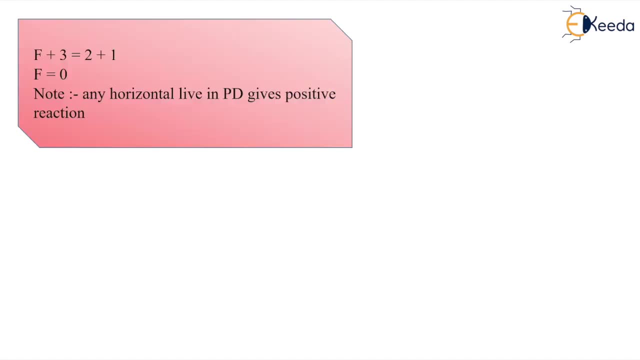 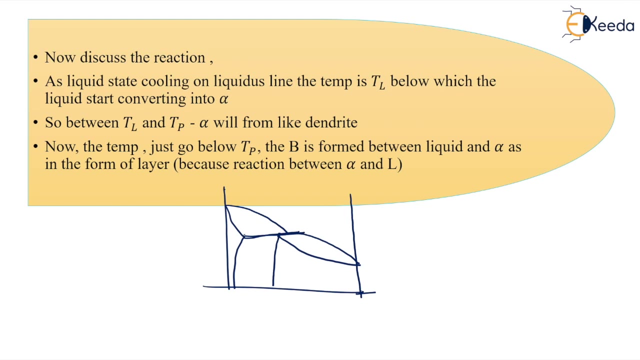 So say, As this liquid starts cooling on the liquidus. So once again, I will draw this, Just, I am drawing the diagram for understanding. So this is liquid, This is alpha. This is alpha plus beta. This is beta. Alpha plus liquid. Liquid plus beta. 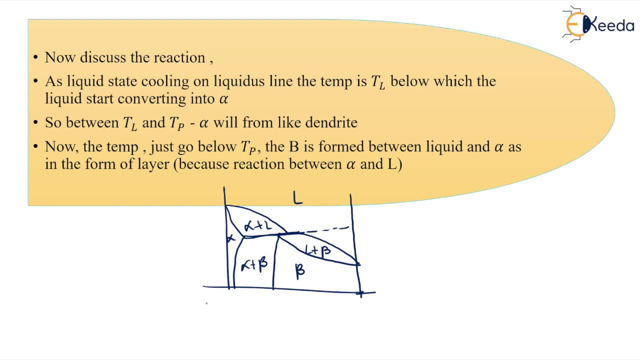 Okay, And this is alpha, And this is alpha, And this is alpha. This is A B. percentage of X in B. This is D A, This is D B. Okay, So, dear students, so what is going to happen here? 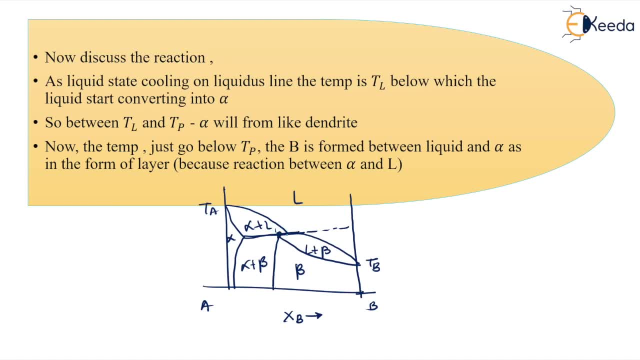 Of course, this is our peritectic point, and this line, horizontal line, will give us the reaction that is liquid plus alpha, undergoing cooling, forms beta. Okay, This is a peritectic reaction. So now, dear students, as liquid start cooling, as see, this liquid start cooling on this liquidus line, on this liquidus line, of course, I am taking this, I am taking, say, this point for the understanding: P point. P, that is peritectic point and the composition at that is X in P. 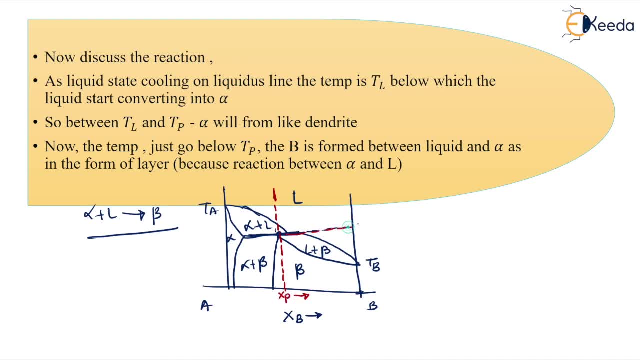 Okay, And here temperature will be. So, dear students, when I start cooling this liquid below this, this liquidus line, below this liquidus line, and the temperature will be what here Say temperature will be, say T, L on the liquidus line. 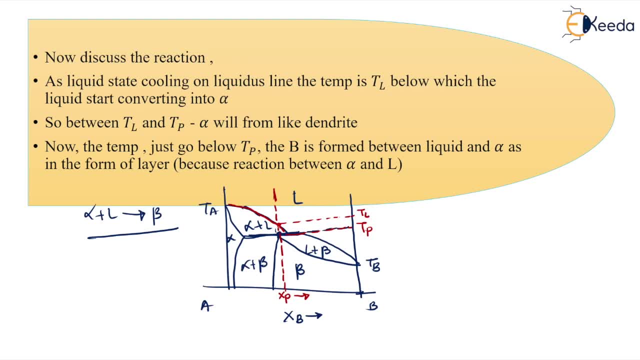 So below which the liquid start curving into what? So, below this, definitely this alpha rich region, isn't it So A rich region? definitely the alpha is the interstitial solid solution. So, as soon as you just come down below this liquidus line, 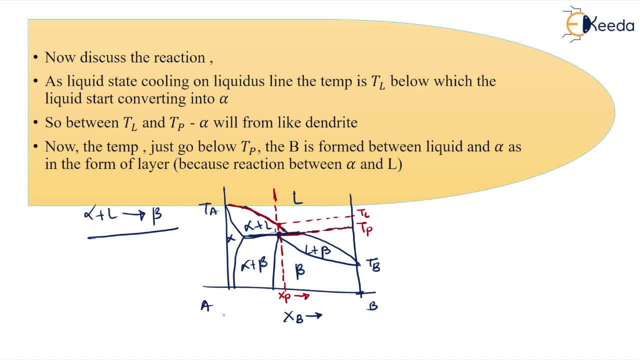 So there there will be the formation of what The alpha And say this alpha is going to start to form. in which manner? From, say T L, from this T L to T P, So just below this liquidus line, alpha start forming. 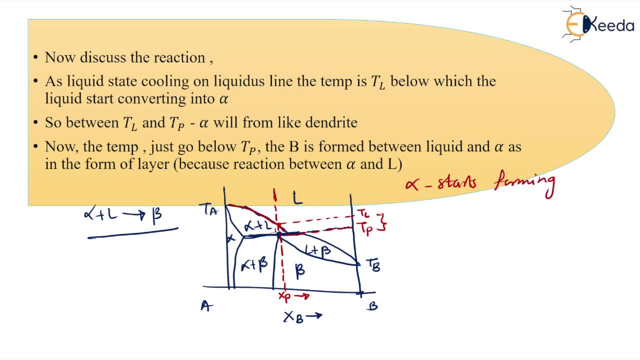 And after nucleation, or after this alpha get formed, it will try to group, Isn't it From where to where? From T L to T P, Isn't it So, dear students? so if I draw here, and very, very popularly, or very basic, we have understand that. 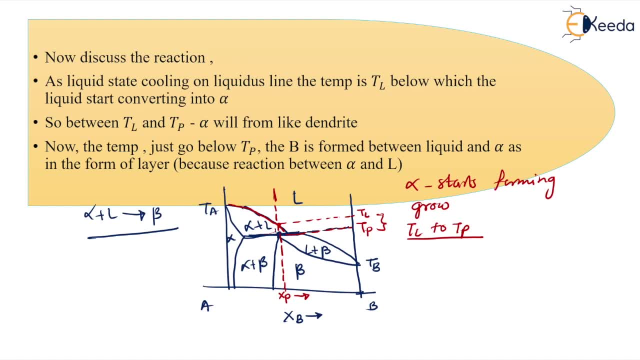 So very easy phase or very easy structure to get nucleate. that is the dendritic fashion, Isn't it? So see, here I am saying that, say, by somehow this alpha, It is getting formed and it get grown like a dendrite. 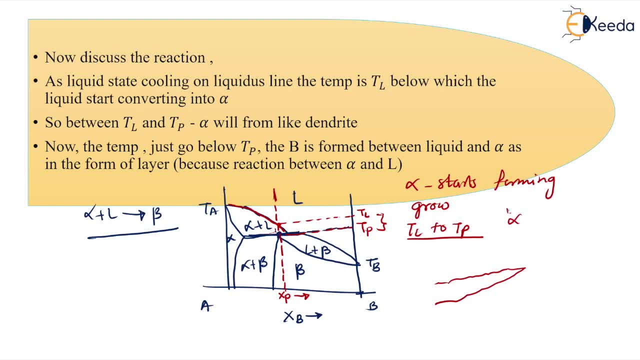 Okay, So alpha grown like. the alpha grow like, grow like dendrite, Dendrite, Dendritic structure. Now, dear students, the temperature just go below this T P, What will happen? So now, from here, just below liquidus, alpha start. 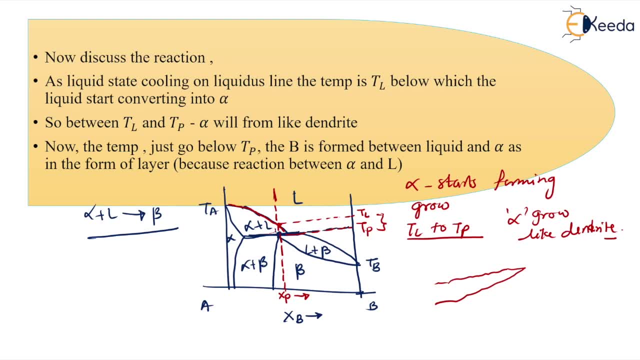 Forming in the term of, say, very common structure, the dendritic fashion, And from T L to T P, it start getting growing, And it is grown in between the temperature T L to T P. Now, dear students, now you just cool again below the T P line. 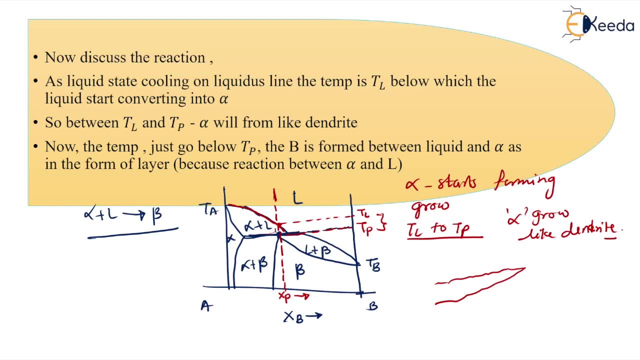 Below this T P, what will going to happen? So definitely the beta is formed between the liquid and this alpha. So, dear students, now you just cool again below the T P line. So definitely the beta is formed between the liquid and this alpha. 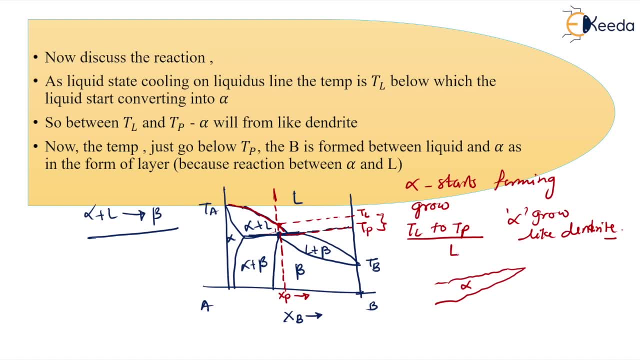 So, dear students, alpha is here, isn't it, And say: here is a liquid. So here is a liquid, It is surrounded with the liquid. Now, just below T P, what is going to form? So definitely so, beta is going to form, dear students. 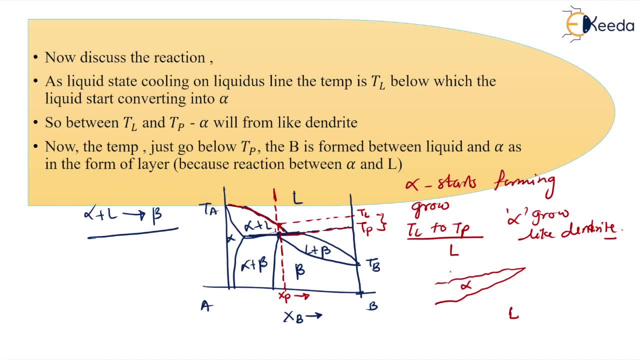 So I will show it with this blue color. So because of liquid, see, because of this liquid plus alpha, this liquid plus alpha just below T P, we are saying, dear students, Now, on this alpha, the beta starts forming. okay. 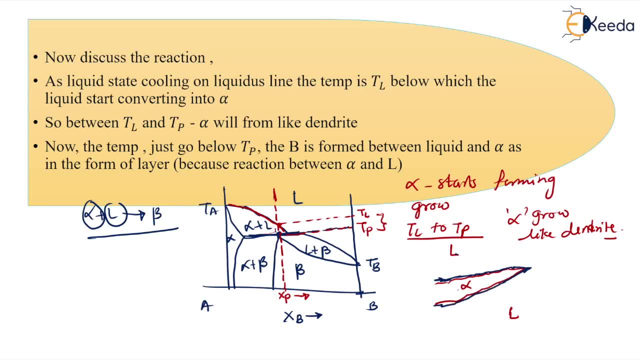 The beta starts forming. okay, So, dear students, beta will going to form the layer because of the reaction between this alpha and liquid beta is formed. Now, dear students, as soon as this beta layer is formed, this reaction is going to stop. 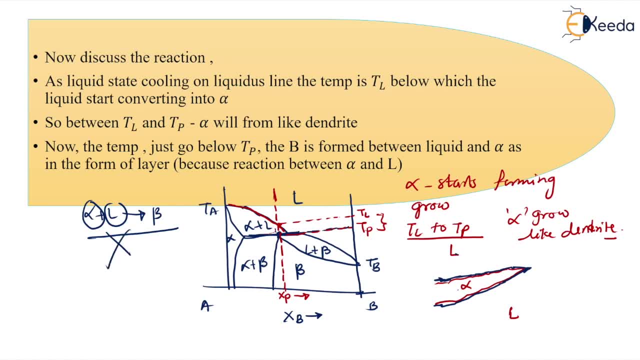 This reaction is going to stop Because the layer of beta is formed on this alpha dendrite. So, definitely, when the reaction is going to stop, so there will not be any further increase of this beta. So this blue color, dear students, is the layer of beta. 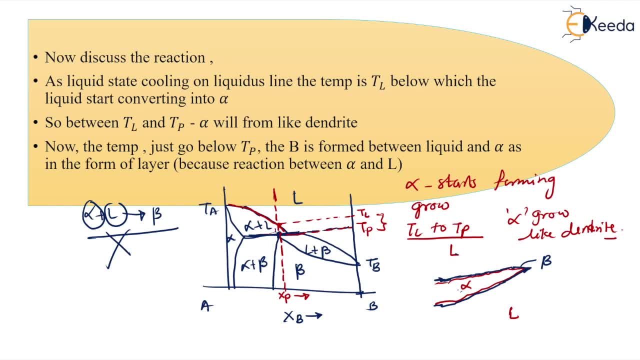 So of course this liquid and alpha is now. they are not directly in contact with each other, Definitely in between them. beta has come So definitely reaction gets stopped, So no more beta is going to Form, dear students. 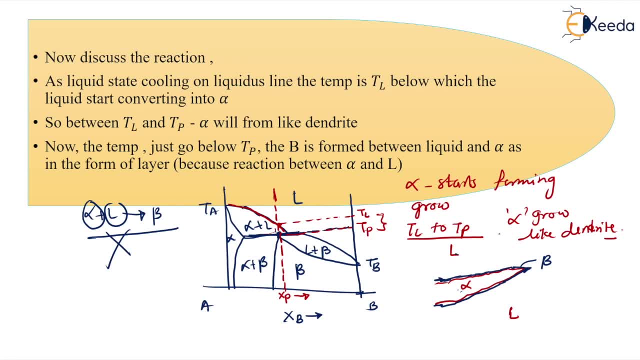 But, dear students, of course, till this reaction is continued, this beta is going to be get bigger and bigger and bigger in the layer form, isn't it? But, dear students, how, when this reaction is stopped, how this beta is going to form. 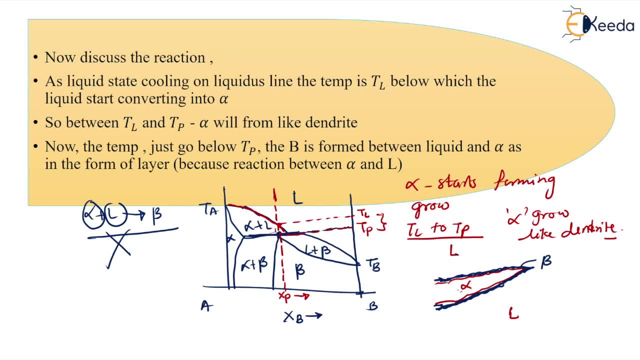 No, dear students, isn't it? Because there should be the direct contact between the liquid and alpha. Alpha was their initial. Now, dear students, here I am saying that once the beta is grown, now, the reaction is completely stopped because of no direct contact. 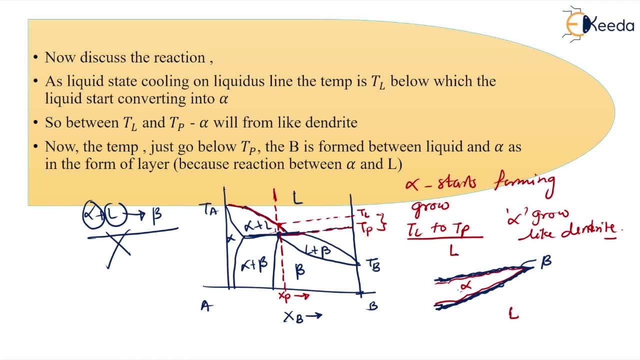 But, dear students, when there is no direct contact between this liquid and alpha dendrite, so this alpha is now going to diffuse. See here, See how this reaction get further continued, How this reaction get further continued Even when the layer of beta is present in between this liquid and alpha. 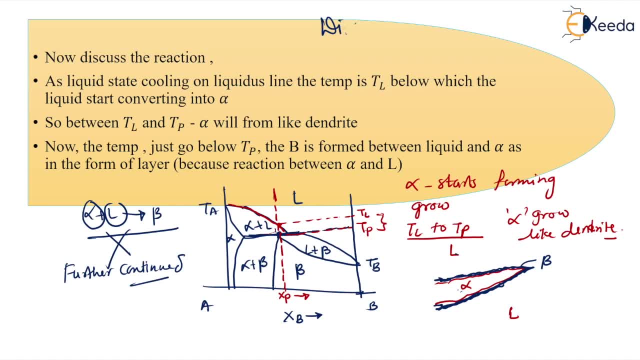 So definitely, dear students, it is because of diffuser, It is because of diffusion, dear students. The diffusion, that is the movement of the mass from the high concentration region to the low concentration region And, of course, this is the function of temperature. 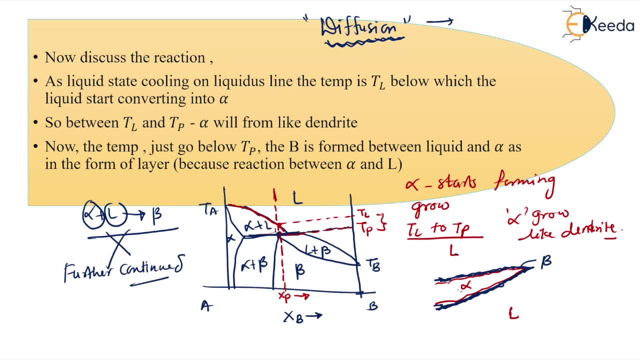 For diffusion we need the temperature. So how this alpha now going to diffuse, How this alpha now going to diffuse Through this layer of beta? this alpha is now going to diffuse through this layer of beta and it is trying to get in contact with this liquid. 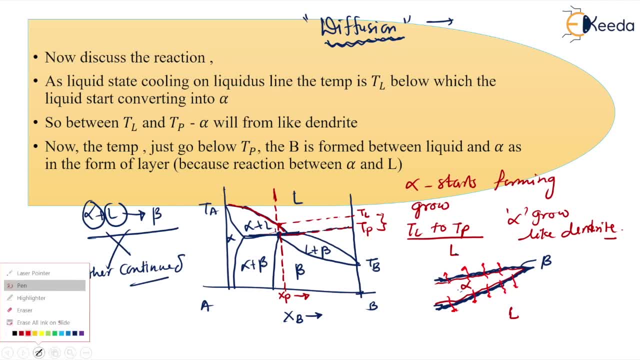 So what is going to happen? So, once again, reaction get started and layer is going to be more and more thicker. Isn't it So like that, because of the diffusion of this alpha through this layer of beta? again, this reaction is get continued, dear students. 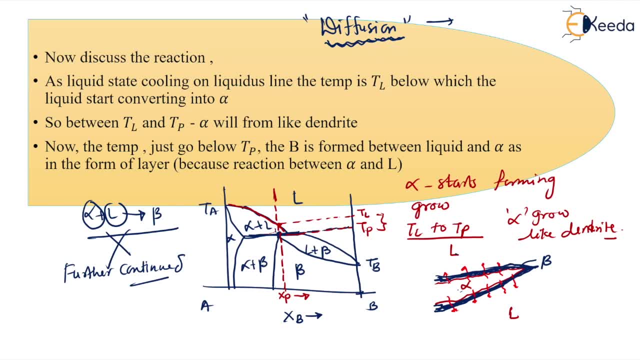 But whether this diffusion is continued for the longer period of time. No, dear students, because diffusion is time dependent phenomena. That is the distance, how much it is gets diffused. x if I say distance, that is how much distance gets diffused, is equal to root of dt. 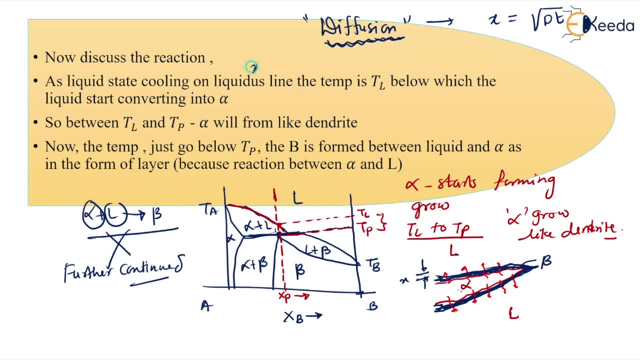 You know this equation very well, dear students. where this x is equal to distance and distance is equal to time, and where, the dear students, d is our what, The diffusivity d is our what. Diffusivity which is equal to d naught into e to the power minus q. divided by this is: 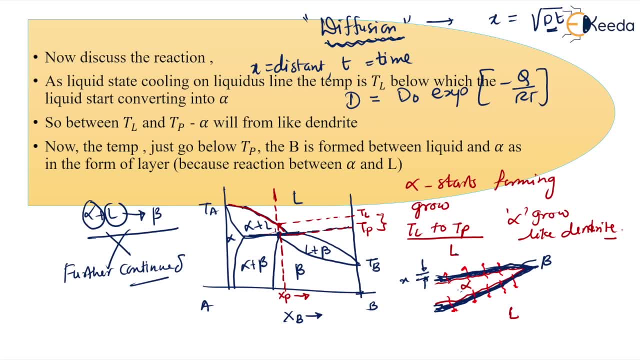 the Arrhenius type of equation for the diffusion, dear students, where we know that that is small d naught is what? The diffusion constant q is the activation energy for this diffusion, that is in calorie per mole. r is the gas constant, that is 1.987 calorie per mole per kelvin, and t is 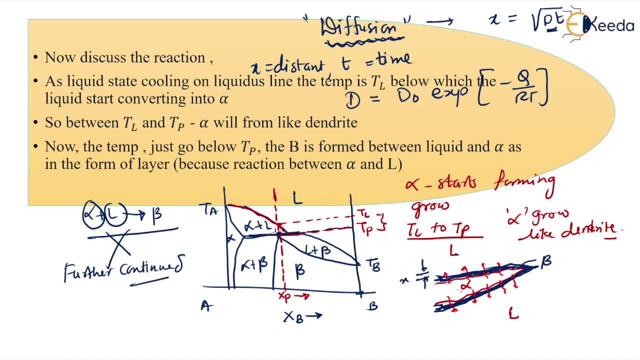 our absolute temperature. okay, just for your information, I am telling So. because of this diffusion, the reaction again gets started and again the beta layer is now growing. but, dear students, how long will this go on for? So diffusion is not like that. it is happening and happening, okay. so this is time dependent. 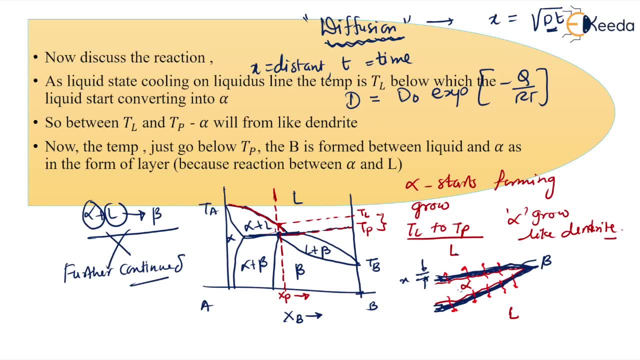 phenomena. Okay, So as a result of this, dear students, what is going to happen? bhale ye reaction, kitni bhi det tak chalegi, lekin at the end kuch na kuch. alpha, kya ho jayega, because see temperature. 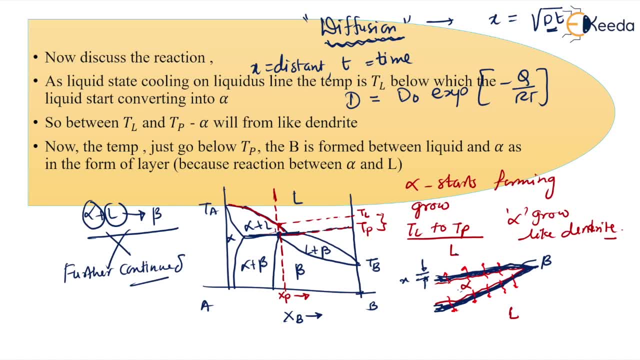 toh definitely, it is having the gradient, so it is definitely reducing, reducing. reducing because we are cooling, it isn't it So? and if a diffusion ke liye, kya chahiye? time chahiye and temperature, isn't it? 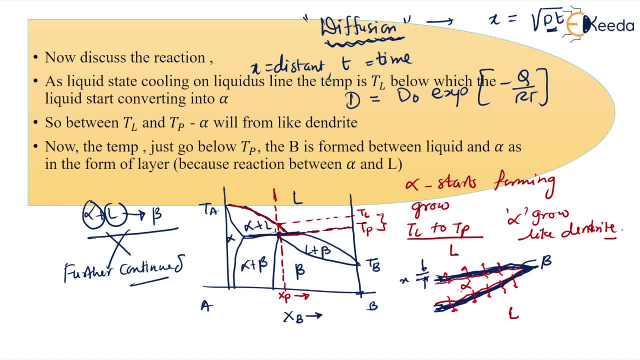 And of course time toh lapse hota rahega, chaise, chaise, cool hota rahega, isn't it? So that is the reason why, dear students, this alpha not completely get converted into this beta, because in between kya ho jayega? ye jo material hai liquid thanda, hote, hote. 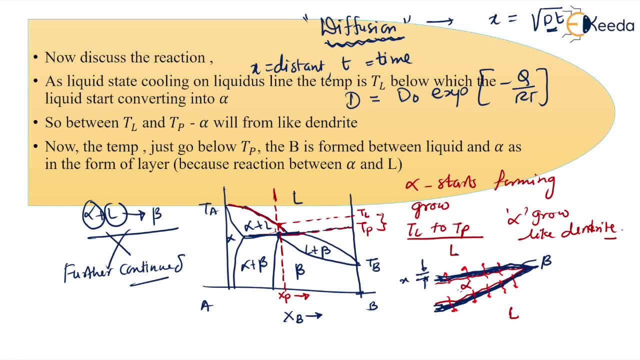 cool, ho jayega, and it will become solid. So actually, what will happen there? some alpha is going to left In this reaction, dear students. okay, so as time increases, this alpha, some alpha is left over in the peritectic reaction and the reaction therefore, dear students, never. 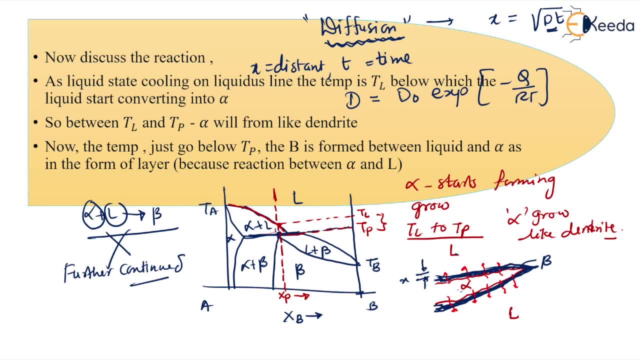 get completed. okay. So it is not like that that 100% alpha is going to convert into this beta. why? Because some alpha is going to be there, because diffusion is a time dependent phenomena and we are cooling it In the material, that metal, continuously to the room temperature. so definitely kabhi. 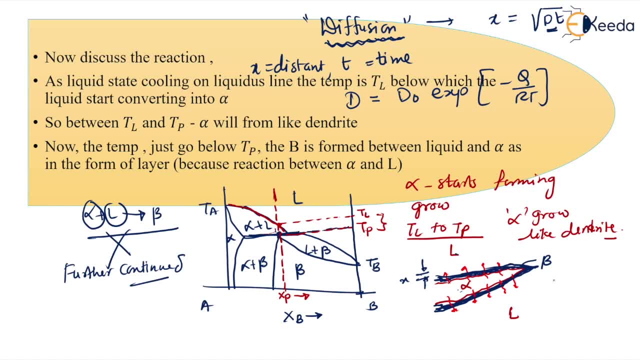 na kabhi. toh ye reaction kya ho jayegi, stop ho jayegi, or ye jo alpha hai. this alpha will get retained in this reaction. this alpha which is retained, dear students, is called as the properitectic alpha. this retained alpha, dear students, please remember this. 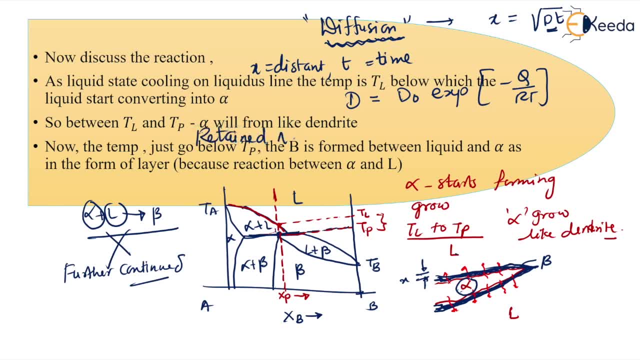 retained Alpha in this peritectic reaction is known as properitectic alpha. which is known as properitectic alpha, dear students. So this is how we can explain the reaction, dear students. Again, dear students, we can take another example, that is niodium, iron and boron. 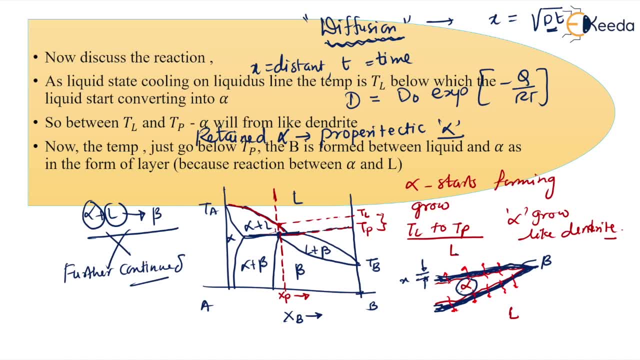 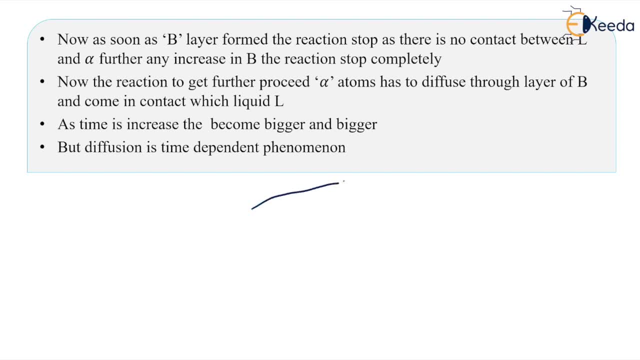 which is the strong magnet. okay, So again in that also, see In that also, dear students, we are having this gamma iron get formed. that is liquid plus. this gamma iron is going to form this niodium, iron and boron phase, which is the 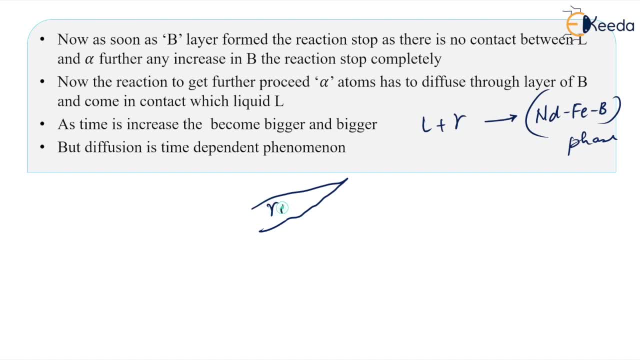 strong magnet, dear students, Here is the gamma iron. okay, and once it react with this liquid, definitely what is going to form? This phase is going to form, dear students. Okay, that is the phase of this niodium ferrous and boron, which is a strong magnet, but what? 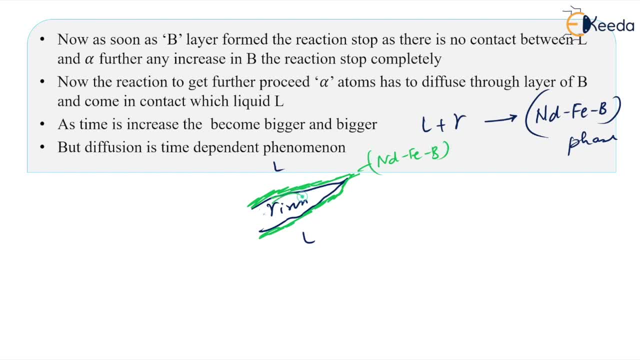 happened Because this reaction never get completed. so some of this gamma iron is going to left in this reaction, okay, and which is not the strong magnet, dear students, this gamma is the where this gamma is going to retain. So at the interstitial 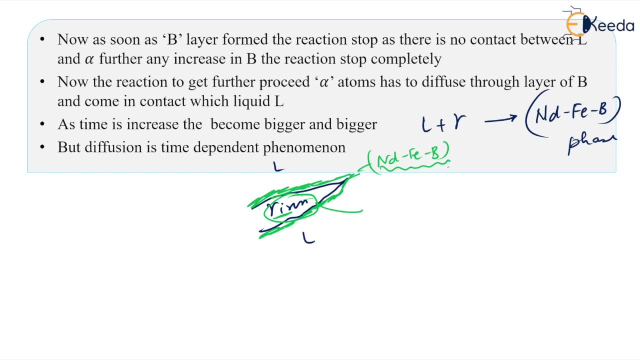 At the interstitial side of this strong magnet. okay, this gamma iron, which is the weak magnet, is going to retain and that results into what One is strong magnet. if I am having one is strong magnet and in that we are having 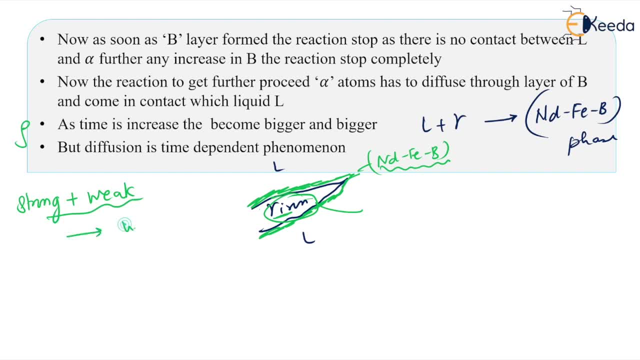 one is weak magnet, so definitely resultant will be what The weak magnet, isn't it? So that is the react. that is the reaction actually, dear students, we are having in this strong magnet. Okay, Okay, Okay. 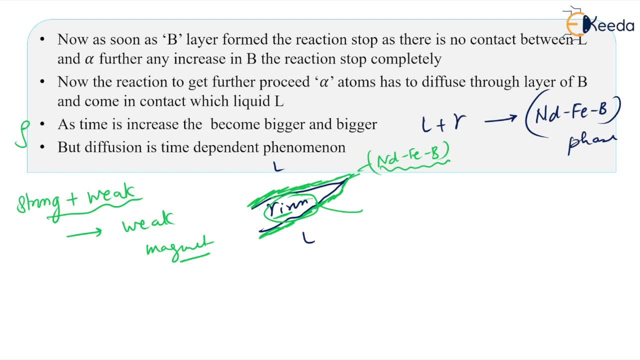 Okay, Okay. That is the reason, my dear students, the China has a very good command on this reaction. that is, this strong magnet is basically used in the headphones and you can see, or you might be knowing, that the China is having more than 95 market shares in these headphones.